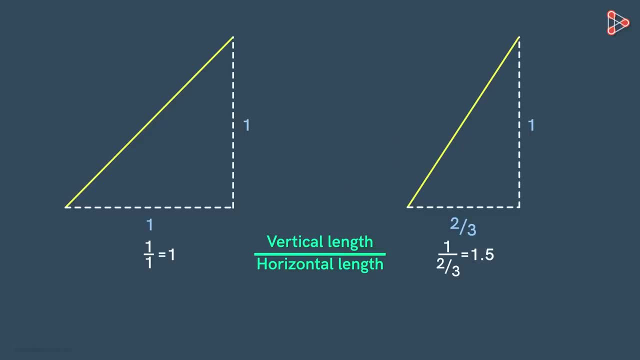 What does this tell us? If we walk along these lines, this ratio tells us how much vertical distance we cover relative to the horizontal distance. So if the ratio is higher, it means that the slant line is steeper. We can also see this as the distance covered while going up. 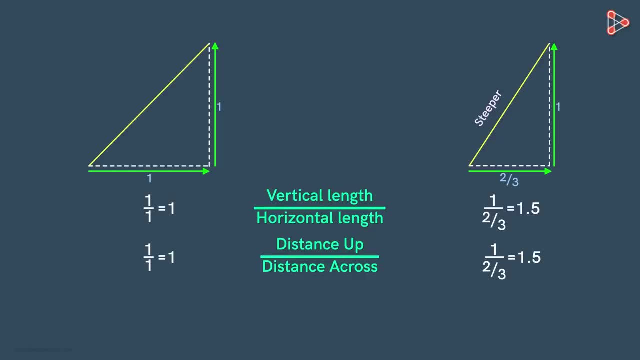 We can also see this as the distance covered while going up, per unit of the distance while going across. There's another way to know which line is steeper, And that is to find this angle Greater, the angle, steeper will be the line. 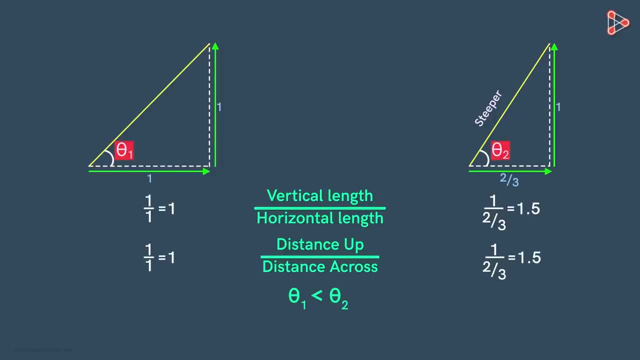 But notice that these two lines are connected to the angle by the trigonometric tangent function. This ratio is equal to tantheta 1 and this is equal to tantheta 2.. Such a ratio for a straight line is called a tangent, Or in English it is called its slope. 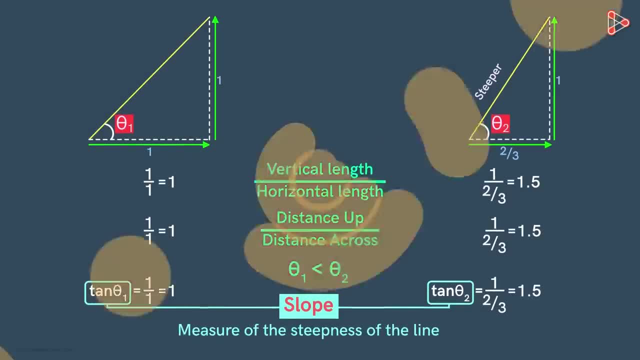 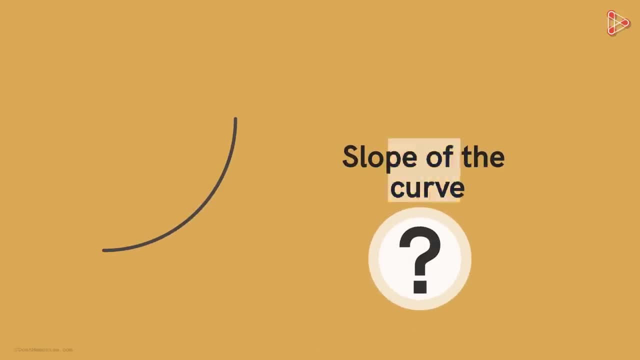 It is the measure of the steepness of the line. Now look at this curve. What is the slope of this curve? Does it even make sense to ask this? What do you think? In this video, we'll understand what this means. 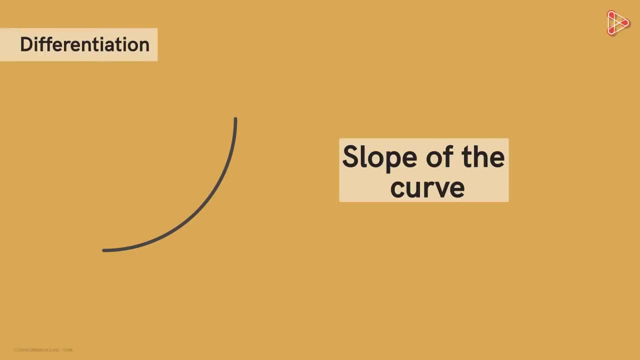 Here the process of differentiation helps us Also. we know that such a curve can be represented algebrically. also we know that such a curve can be represented algebrically by a function between two varying lines. Also we know that such a curve can be represented algebrically. 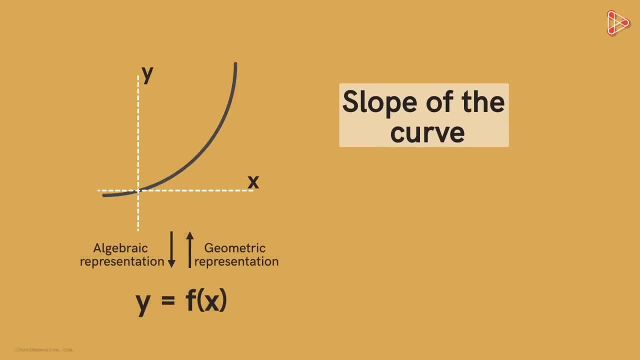 variables, We will see that this slope is connected to the idea of the derivative of a function. So let's continue with our question. One thing we can clearly see here is that different positions of the curve will have different steepness. We can intuitively see that as we move from the left towards the right along the curve. 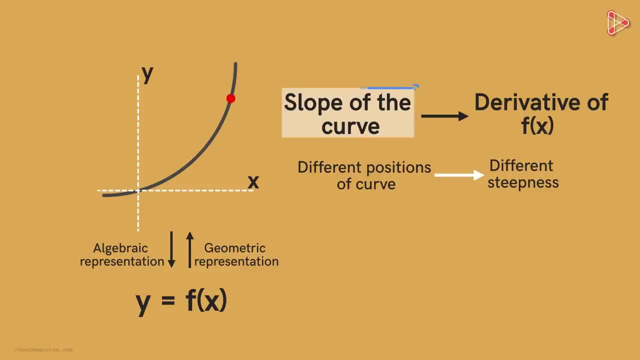 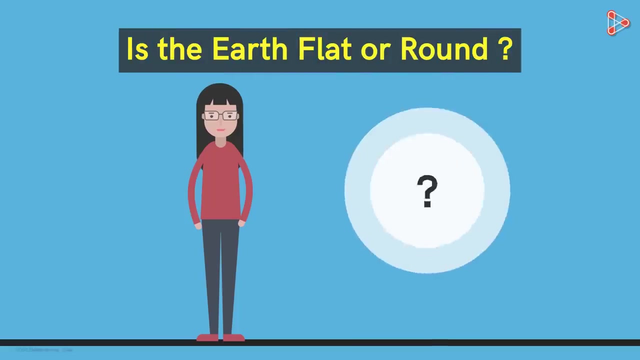 it gets steeper, So the slope of the curve in general doesn't make sense. So let's focus our attention around this point P. What will be the slope at this point? For this, let me ask you one question: Is the earth flat or round? 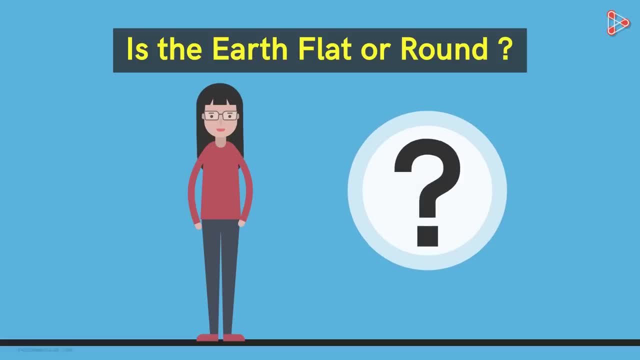 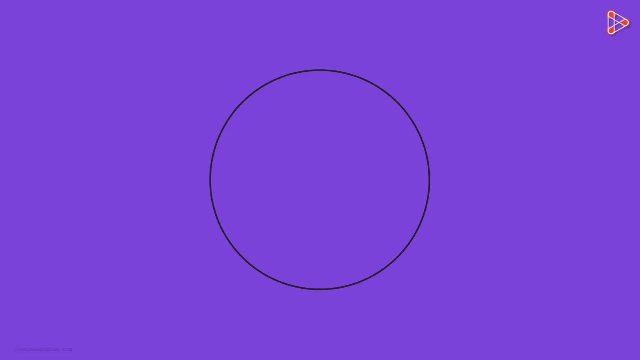 You'd probably be laughing, because we all know that the earth is almost round in shape. But notice the surroundings around you. It seems that the earth is flat. Why is it so? Consider this slope. Let's consider this circle as the representation of the earth. 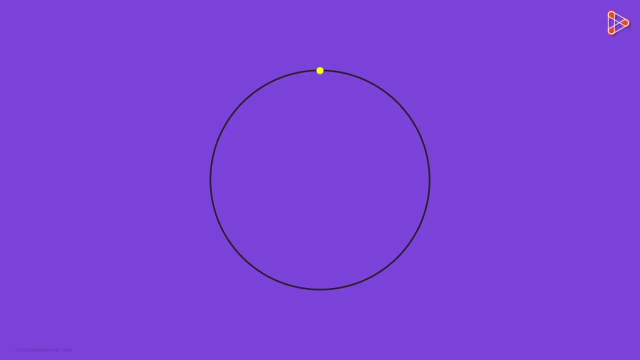 And let's say you are currently situated here. If we zoom in around this portion of the curved line, we see that it becomes less and less curved. It looks almost like a straight line. So let's say we draw a straight line, only intersecting the curve at this point. 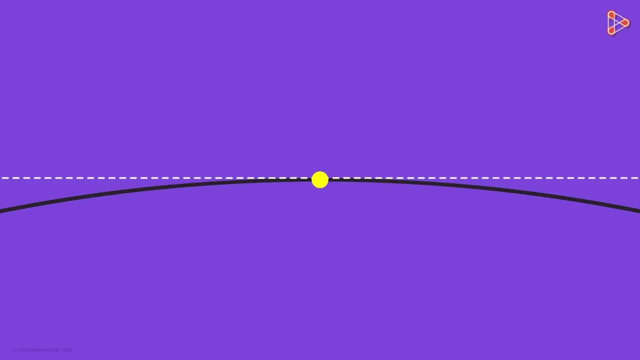 We can see that the curved line is almost the same as this straight line. We know that this line which passes through the curve is the straight line Which passes through only one point of the curve, is called the tangent line. at that point, 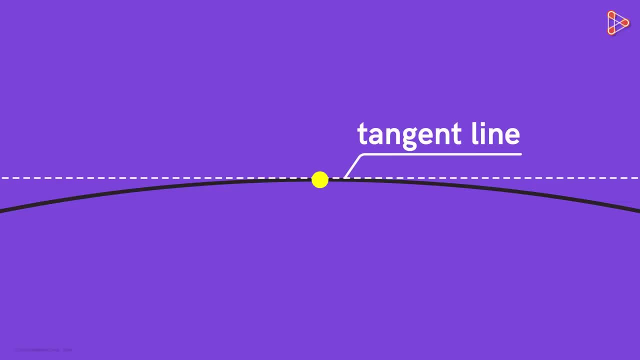 Take a moment and just observe what we found. This is the most important idea on which calculus is built. A curved line in a very small region around a point on it can be approximated by a straight line. This straight line is the tangent line at this point, 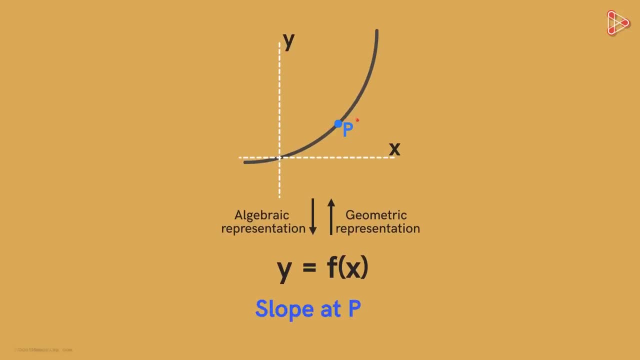 So this solves our problem. The slope of the curve at a point will be equal to the slope of the tangent line at that point, And we are familiar with how to find the slope of a straight line. So how do we find the slope of the tangent line at this point? 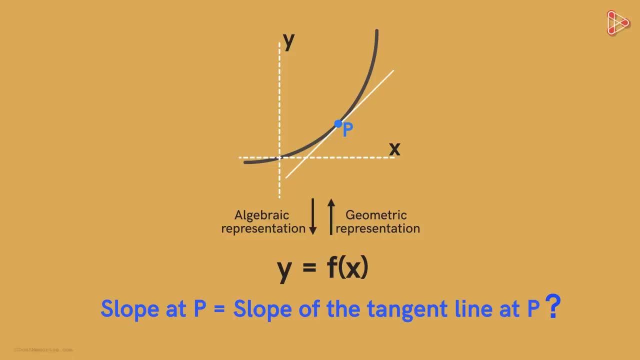 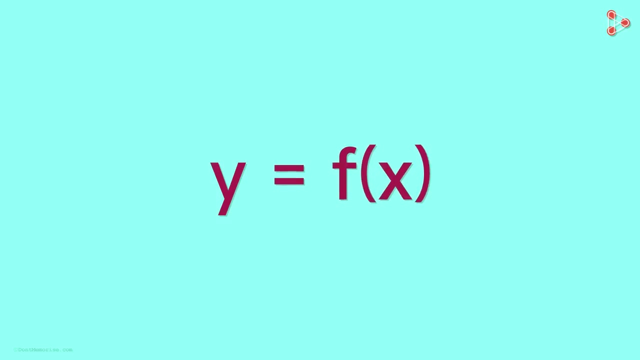 But before answering this question, let's look at why are we so interested in finding the slope? We will continue this in the next part. Previously, we saw what we meant by a function between two variables, x and y. A function tells us how the value of one variable depends on another variable. 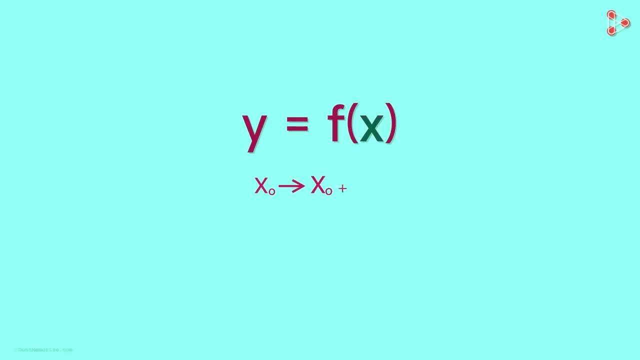 So if the value of x changes from x nought to x nought plus delta x, then the value of y will also change from y nought to y nought plus delta y. Now look at this ratio: Delta y over delta x. 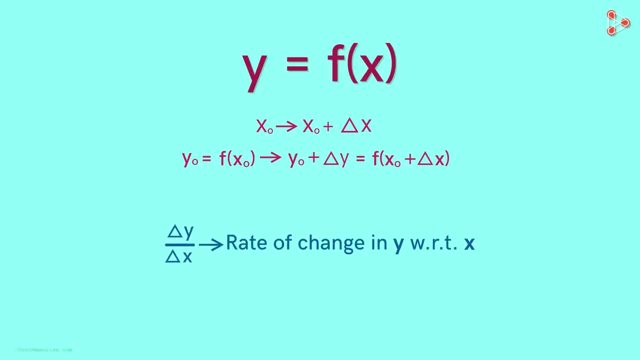 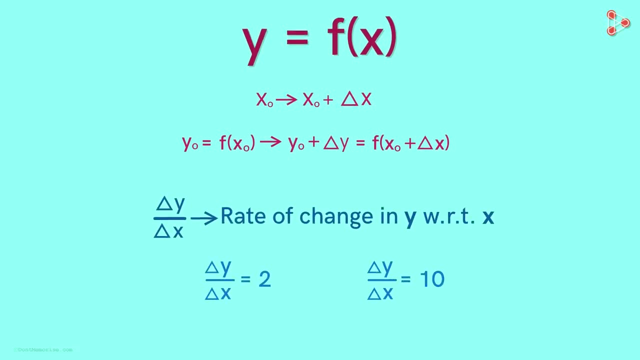 It tells us the rate at which the value of Y changes in proportion to the change in X, For example. consider these two ratios. As the ratio in the second case is greater, the value of Y will change relatively faster. here This rate of change for a function is actually related to the slope of a curve. 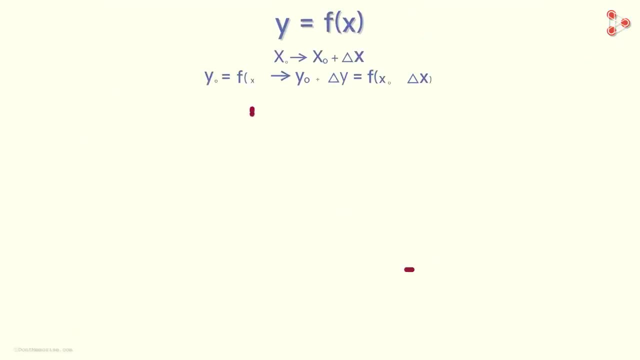 Let's see how Let's say, the graph of this function is a straight line like this: X, not, Y, not is this point. and when the value of X changes by delta X, we reach this point. Now consider the ratio delta Y over delta X. 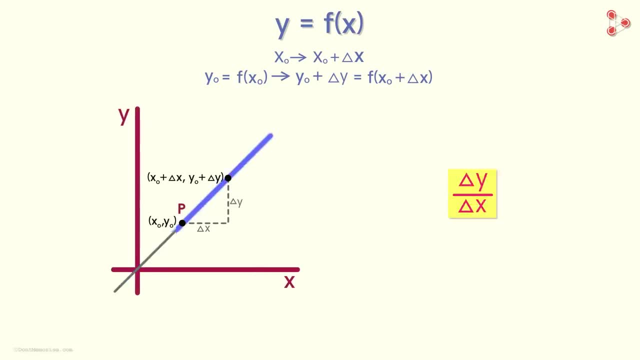 We saw earlier that for a straight line, this ratio is the measure of its steepness. So the rate of change in Y with respect to X is equal to the slope of this line. Now we can see that for a straight line its slope is constant throughout. 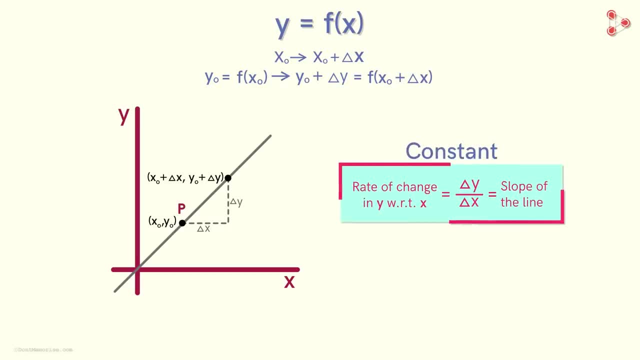 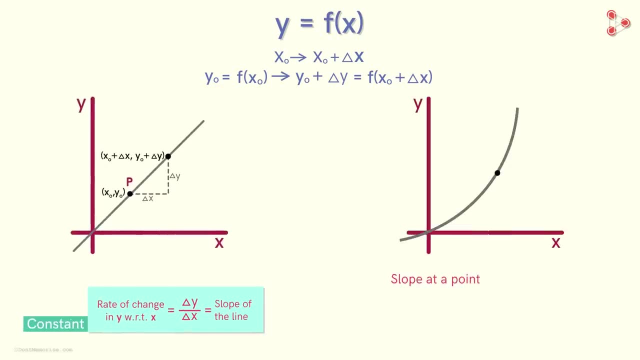 So its rate of change will also be constant. But what if, instead of this, the graph of the function is given by a curved line? The slope at a point tells us the rate of change at that point. We've seen earlier that in a very small region, around a point, the curve can be thought. 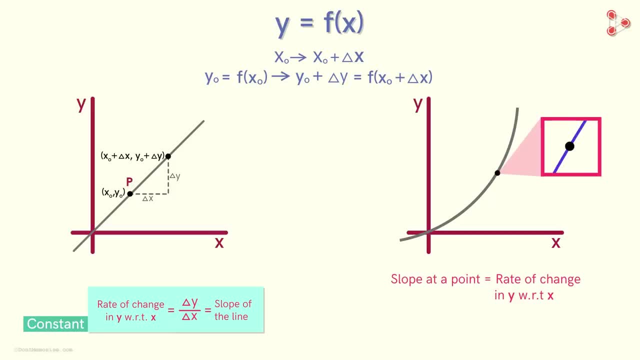 of as a straight line. This is the tangent line at this point. So we see that the slope of this line is equal to the rate of change here. But now we can see that, depending on the point on the curve, the slope will change. 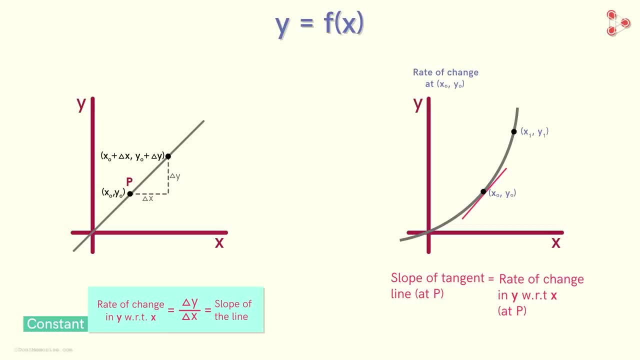 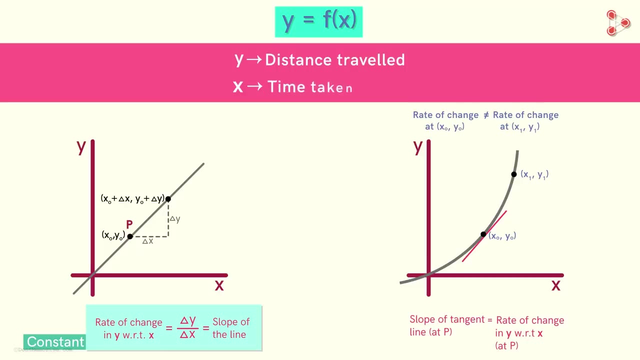 So this means, depending on the value of the X variable, the rate of change will also vary. Now let's look at an example to understand this. Let's say: in this function, Y is the distance travelled by an object in motion And X is the time taken for the distance travelled. 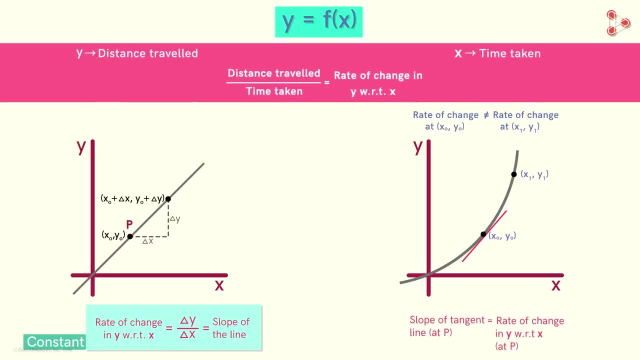 Then the rate of change in Y with respect to X will be equal to the speed of the object. In the first case, we know that the rate of change is constant, So the speed of the object will be constant throughout its motion, While in the second case the rate of change is not constant. 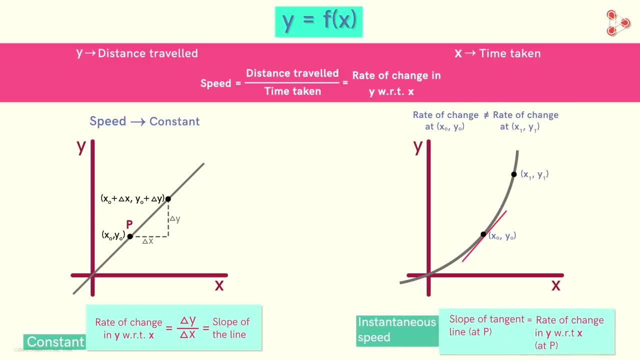 So here this rate will tell us the instantaneous speed of the object. So the rate of change in Y is equal to the speed of the object. For this reason the rate of change for a function at a particular value of X, X nought. 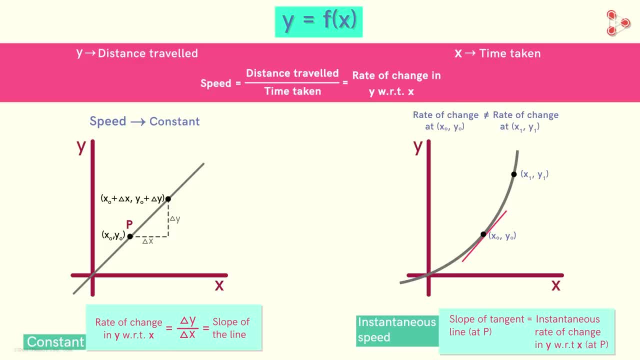 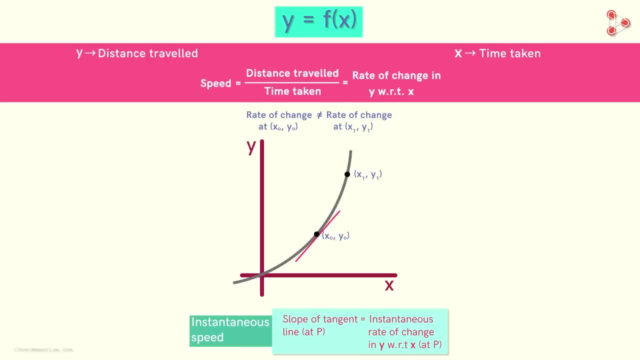 is called as the instantaneous rate of change at X nought. So to conclude, a very small portion of a curve around a point can be approximated by the tangent line. at that point, The slope of this tangent line tells us the instantaneous rate of change of the function. 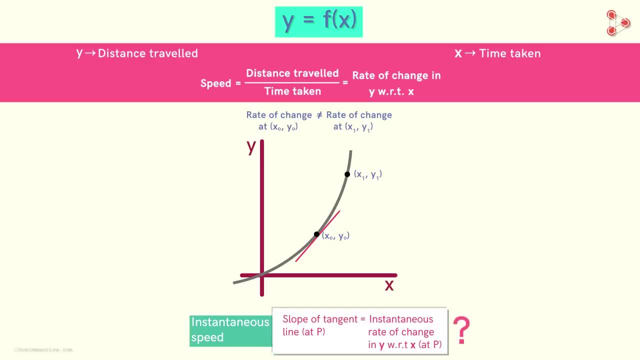 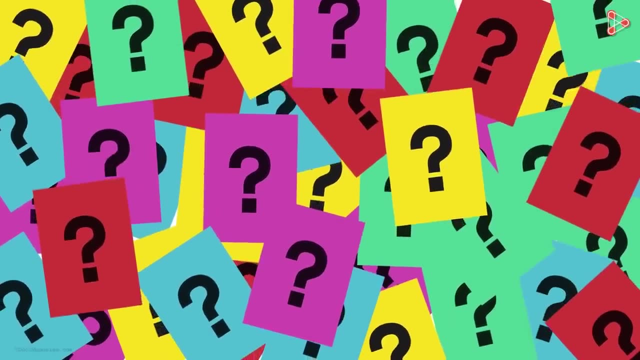 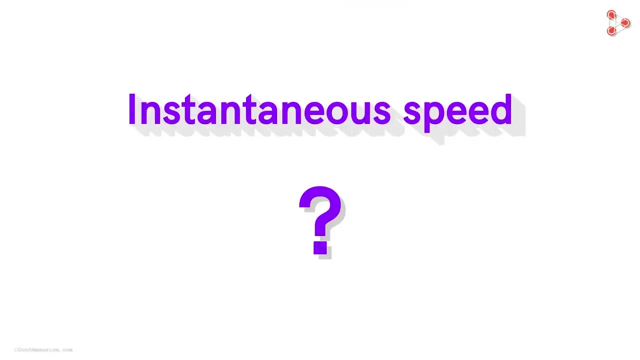 at that point. But how do we find this slope Or instantaneous rate of change? Do you remember that in one of our previous videos we found the instantaneous speed of an object? To find the instantaneous speed, we have to use the process of differentiation. 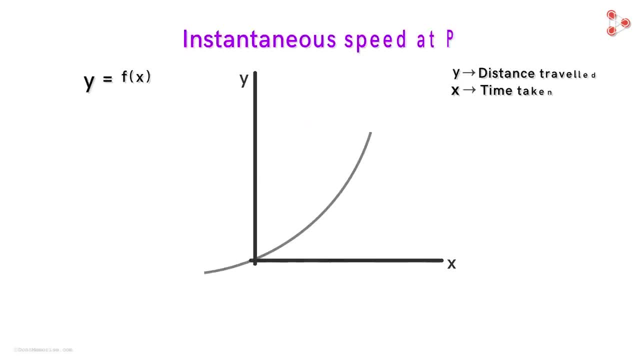 Let's say we want to find the instantaneous speed at this point P, that is, at the time instant X. nought For this we first find the average speed for some time. interval delta X. At X: nought. we find the average speed for some time. interval delta X. 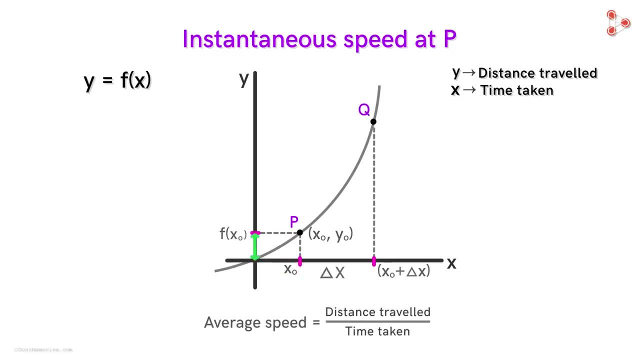 At X nought, the distance covered will be this, And at X nought plus delta X, it will be this. So the average speed in the time interval delta X will be equal to this. For a function, this ratio is called as the average rate of change. 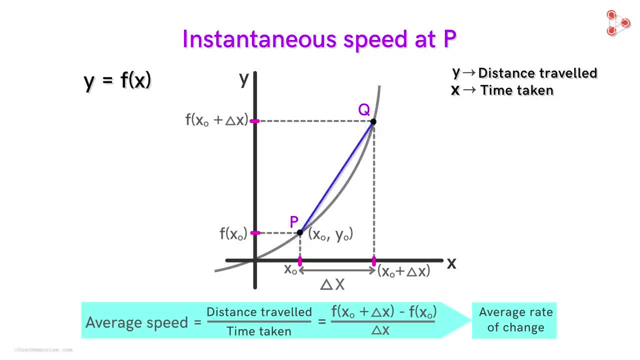 Now let's say we draw a straight line between these two points. It's called the secant line. We see that the slope of this secant line will be equal to the average speed of the time interval, delta X. So we see that the average rate of change between two values of X is equal to the slope. 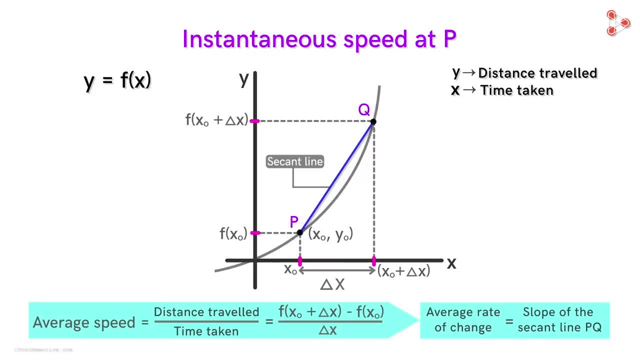 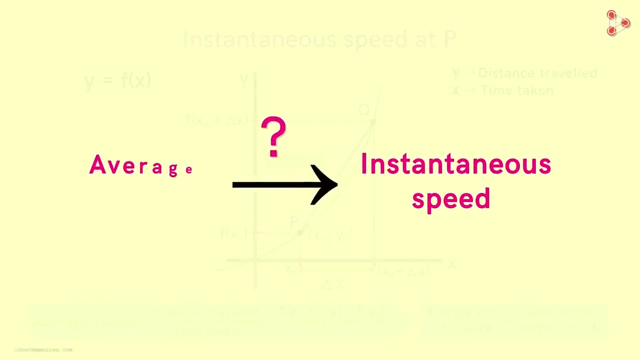 of the secant line between the corresponding points on the curve. Now what's the next step? How do we find the instantaneous speed from this average speed? For this we find the average speed in shorter time intervals, That is, Delta X tends to zero. 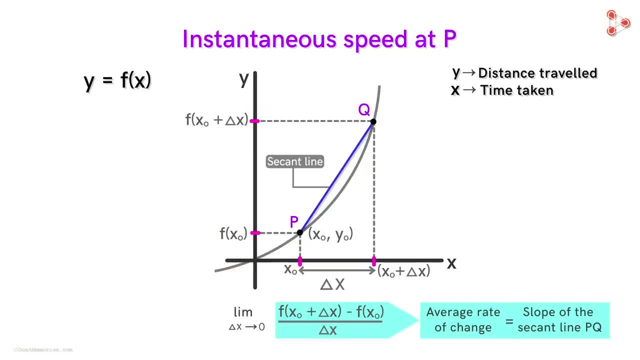 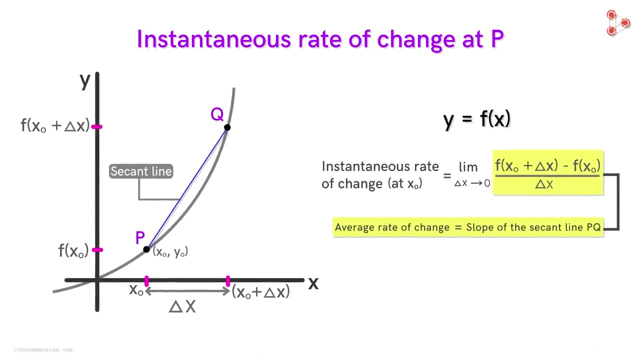 We say that when the limit delta X tends to zero, the average speed approaches the instantaneous speed. This instantaneous speed is the instantaneous rate of change at X. nought Now what happens to this secant line as delta X tends to zero? Let's say we find the average rate of change between points P and Q1,, Q1,, Q2,, Q3,, Q4,, Q5,. 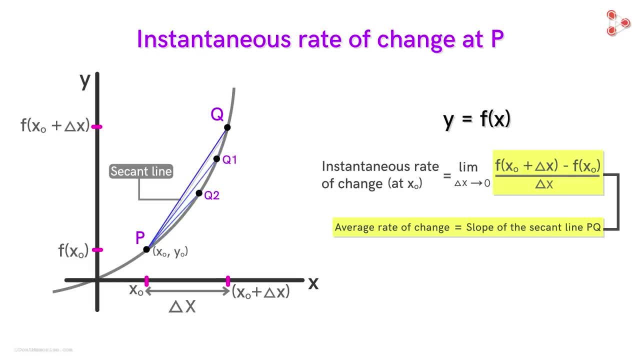 Q6.. We can see that as delta X tends to zero, these points come closer and closer to the point P. So as the limit, delta X, tends to zero, the secant line will pass through only one point P on the curve That is, the secant line approaches the tangent line.